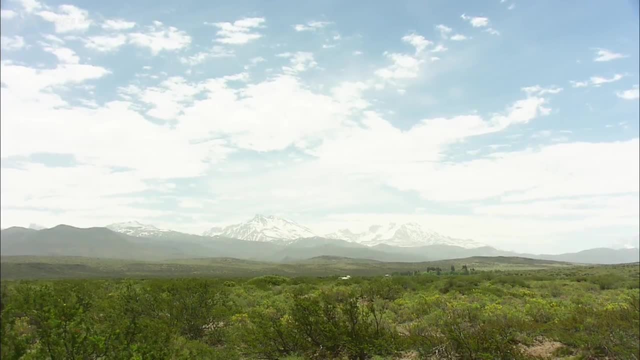 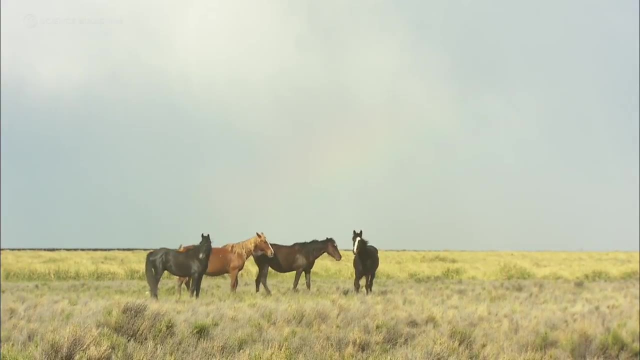 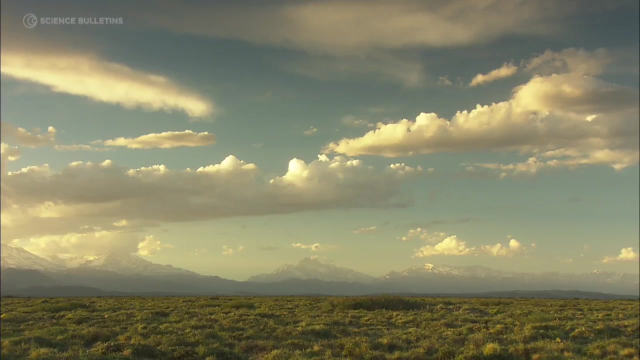 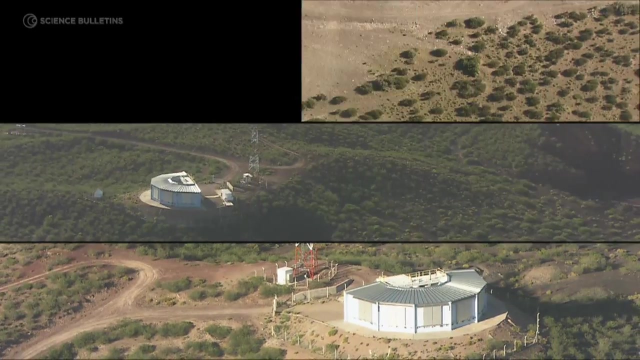 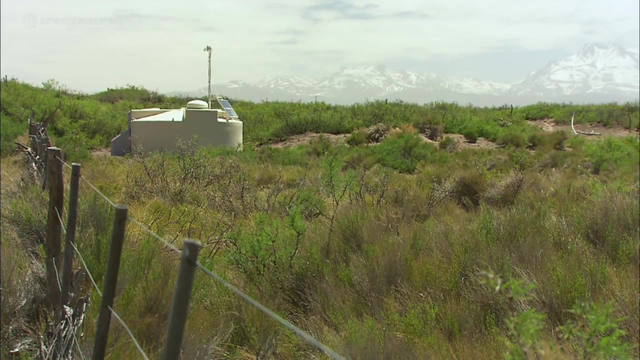 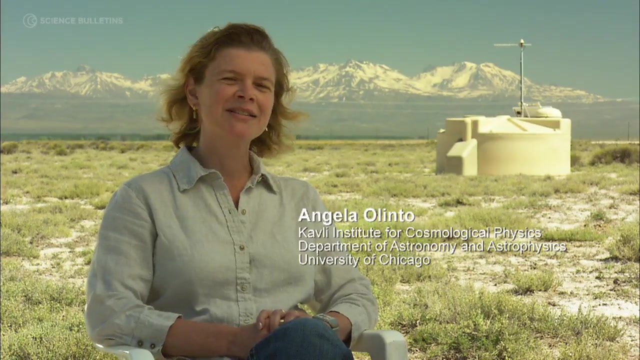 It might not be so obvious that in the middle of this beautiful field, some of the most interesting science is being developed. The Pierre Auger Observatory is a 3,000 square kilometer array of detectors that 17 countries and 300 physicists built to try to understand the origin of the highest energy particles. 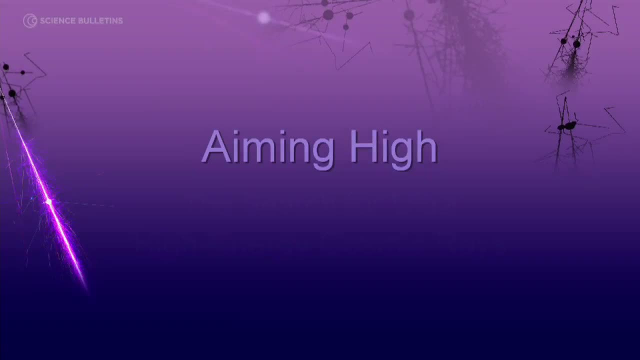 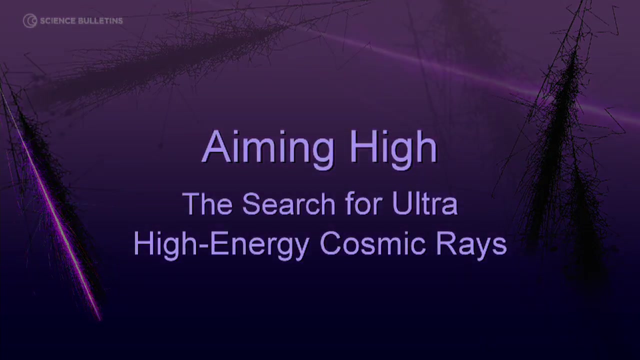 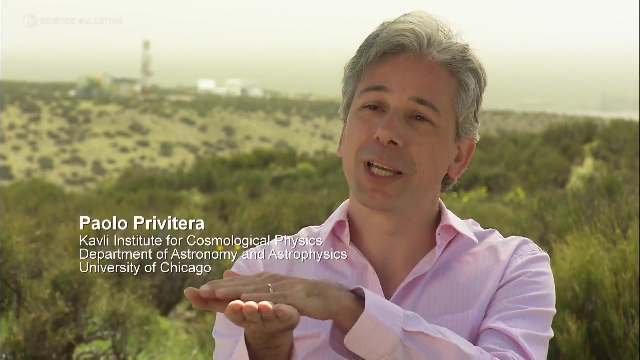 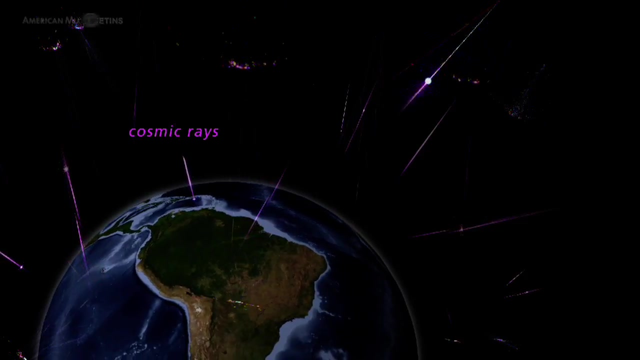 that we've ever observed. Cosmic rays are particles which arrive from the universe continuously on Earth. Right in this moment, through my hand, you have several per second. The one that we are interested in in the Pierre Auger Observatory have 100 billion times the energy of this normal. 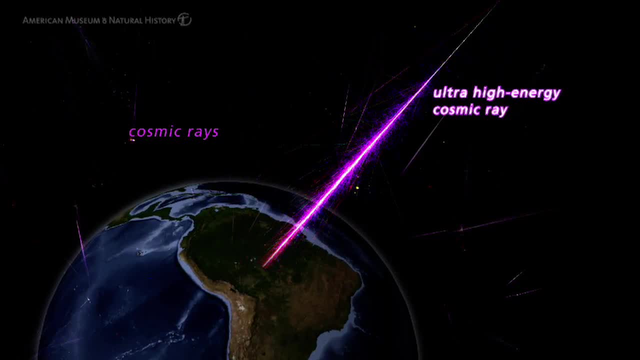 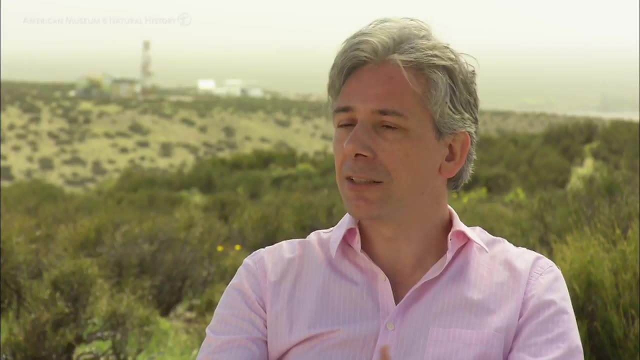 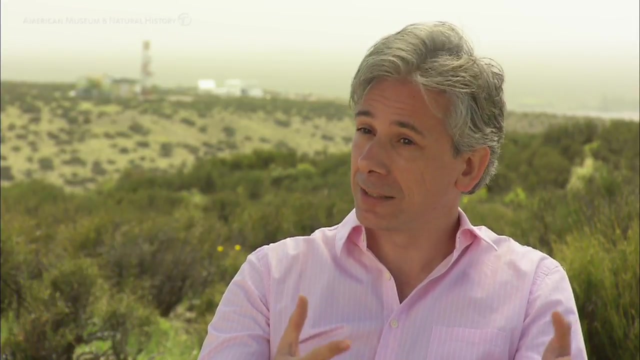 cosmic rays that are passing through my hand. The problem is that it's very difficult to find an explanation of their existence. It's very hard to find a physical process that either generate or accelerate particles at this enormous energy. So what we try to do, 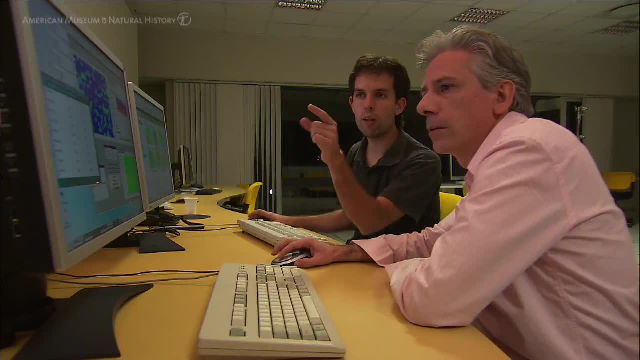 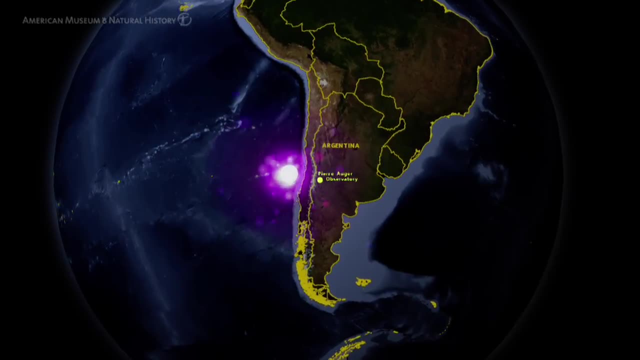 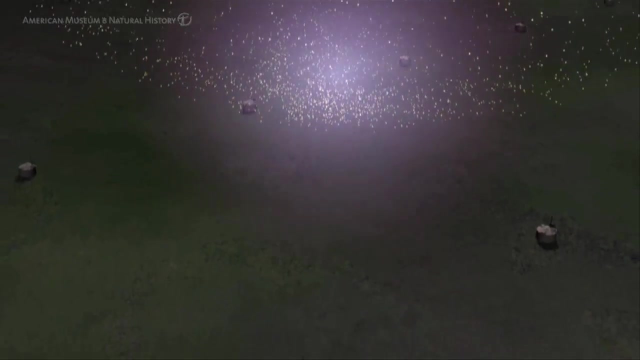 here is to find their origin. But ultra-energy cosmic rays are very rare. You would have to wait 10,000 years to have one landing on a baseball field. So this is why you need a giant observatory like the Pierre Auger Observatory. 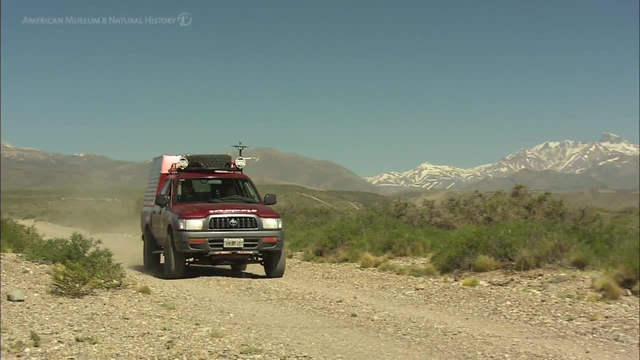 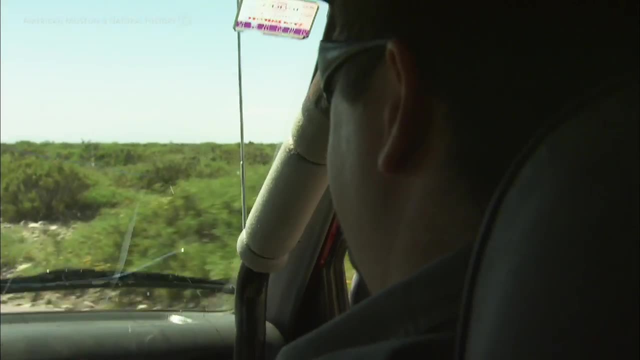 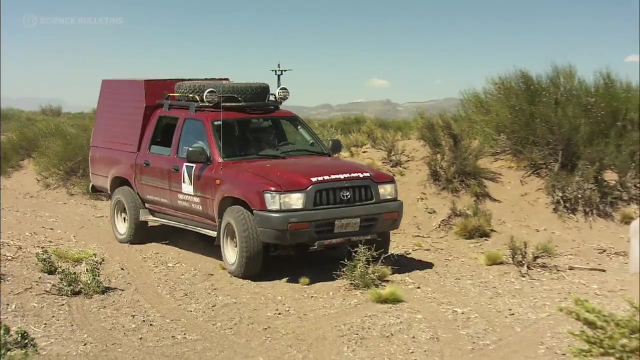 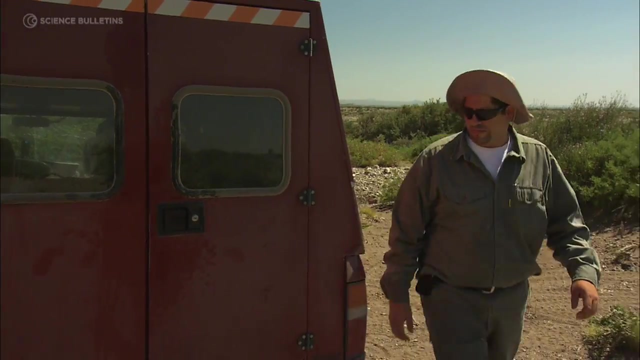 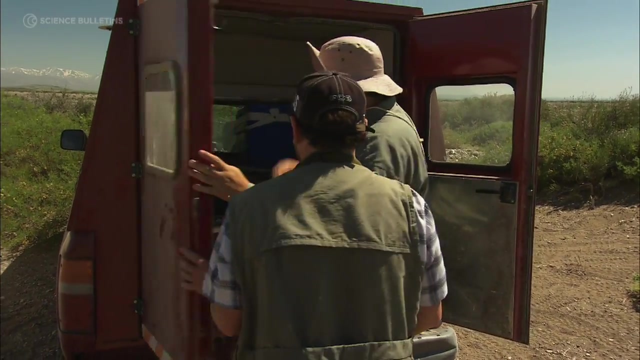 The reason we use this area is because it has the perfect height. It's a very flat region And the population is very friendly to us and is able to let us into their land to leave our detectors. We are electronics technicians, Oscar and me. What we do is maintain the detector. 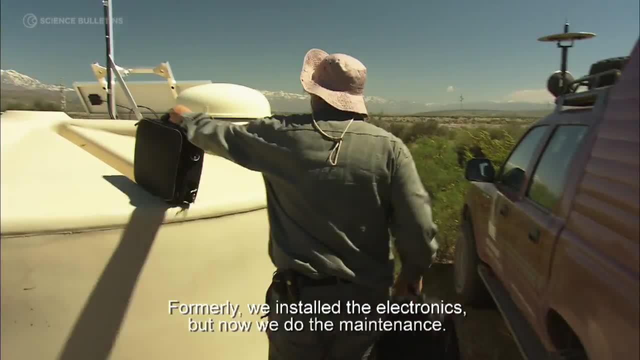 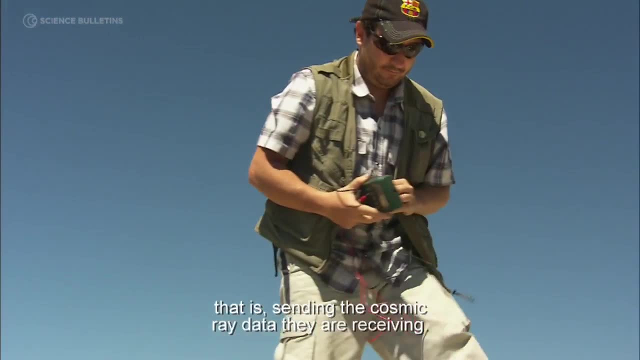 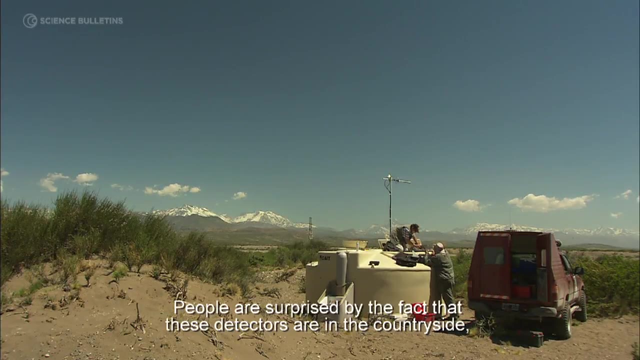 in the field and make it work. Years ago what we did was install the electronics And now what we do is maintain and make the detector work, that is to say, sending data about the cosmic rays that it is receiving. They are very interested in having these detectors in the field That they are not connected to. 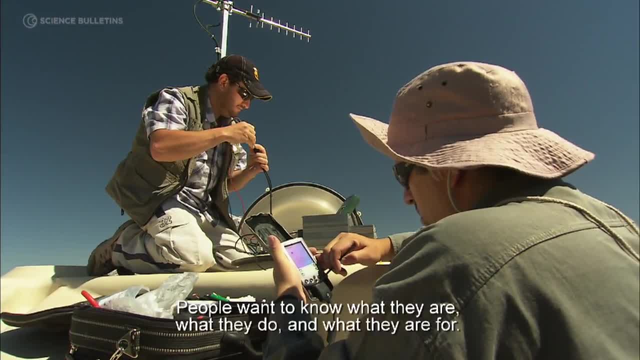 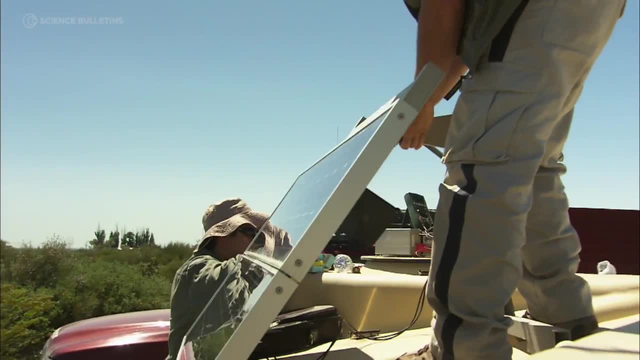 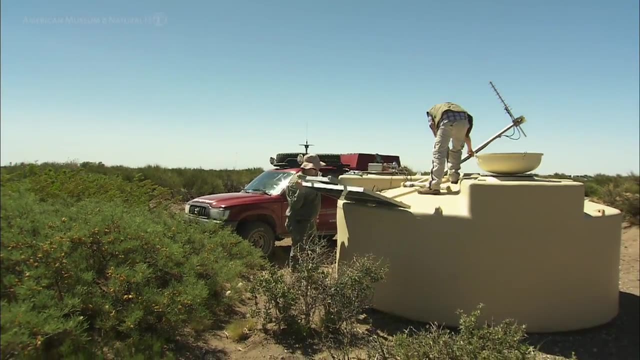 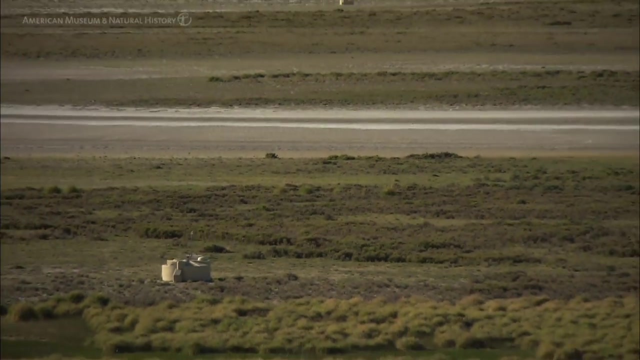 that have a solar panel, that have water inside. They are very interested in knowing what this is for, what this is all for. Well, the Pierogé Observatory is unique because it puts together two different detection techniques. One is based on the measurement of particles at ground. 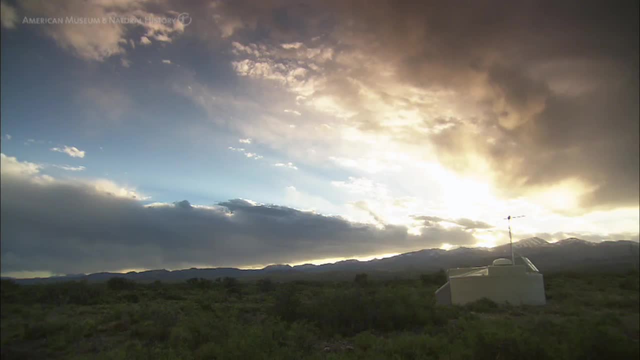 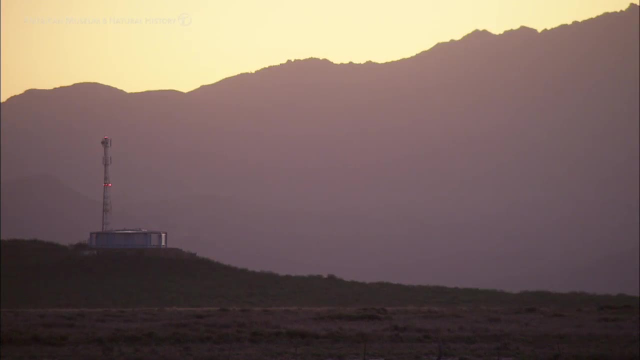 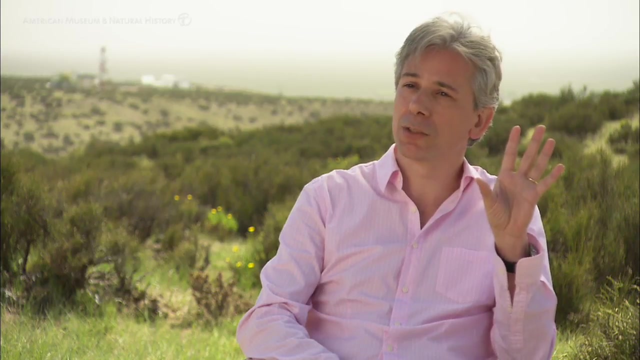 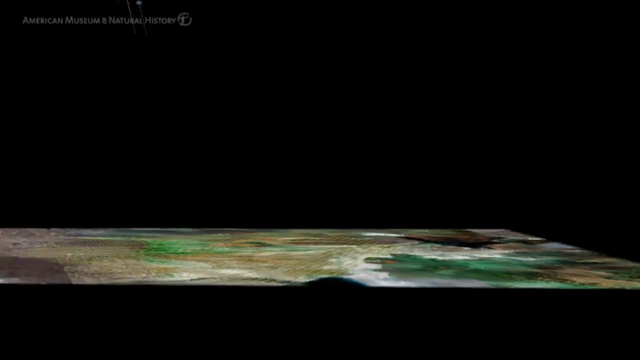 so you have 1,600 detector tanks placed over an area of 3,000 kilometres And you have 24 telescopes that look at the fluorescence light which is emitted by these ultra-high-energy cosmic rays in the atmosphere. So the two systems work together in this way. 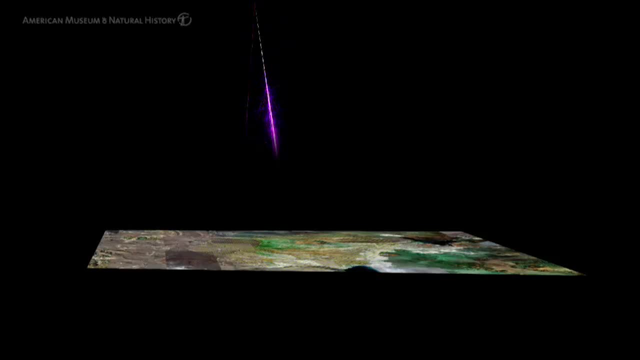 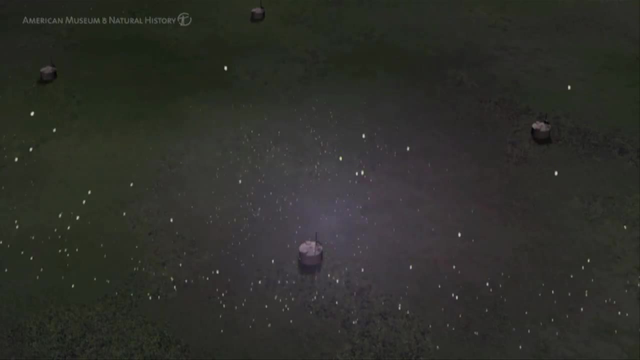 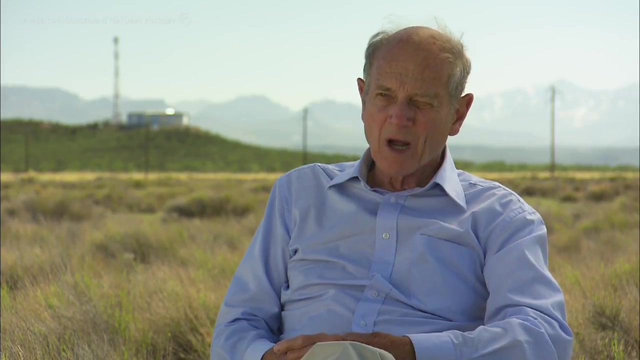 Once one of these cosmic rays arrives from the top of the atmosphere, it produces a shower of particles detected by the surface detectors. In the meanwhile, the shower produces fluorescence light which is measured by the fluorescence detector. The ground detectors measure very carefully the time of arrival of the particles. 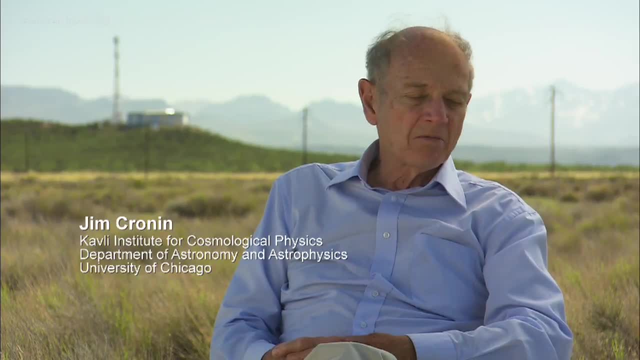 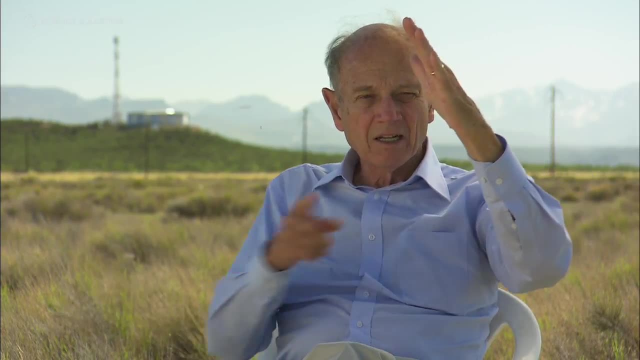 And you can imagine if we have two tanks separated by a mile and a shower of particles, it's really a flat pancake comes down. You'll hit this detector first and this one later. We measure the time difference. do a little trigonometry. 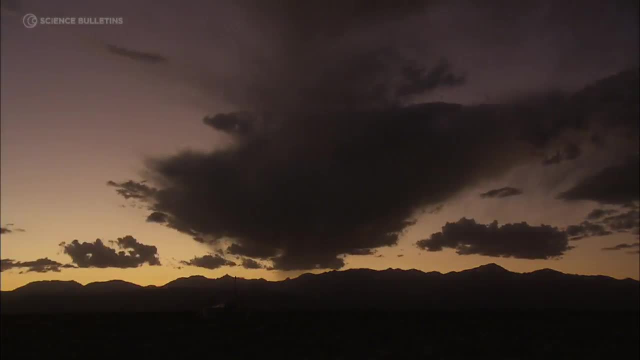 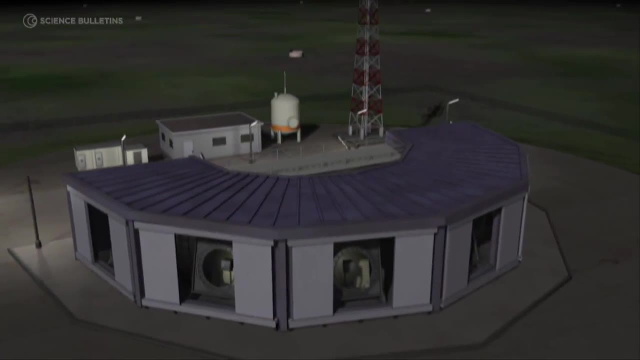 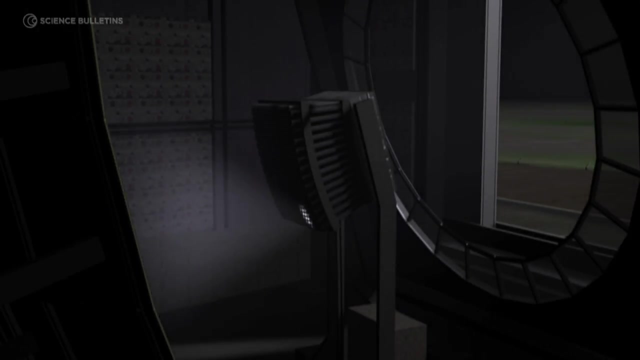 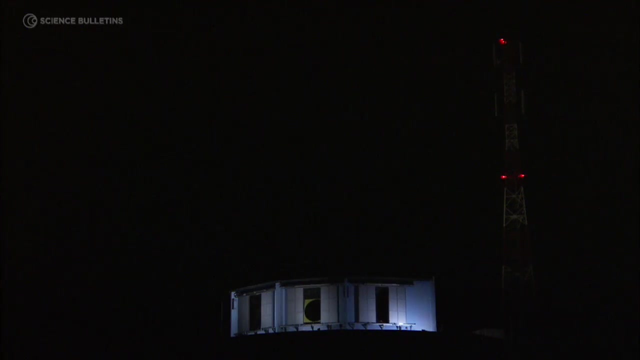 and we have the direction of the particle. The fluorescence detector is a telescope which concentrates the fluorescence light into a camera. Basically, you make a movie of what is happening in the sky. but it's a very fast movie because we make pictures each tenth of a millionth of a second. 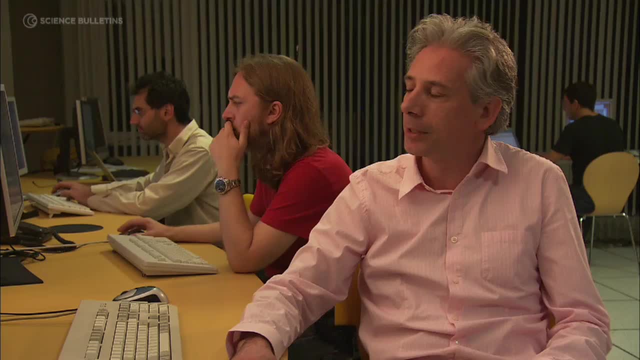 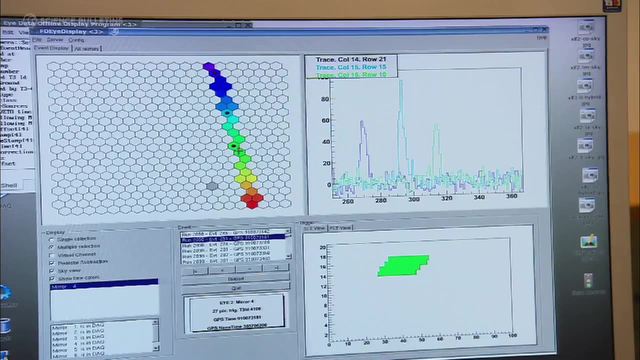 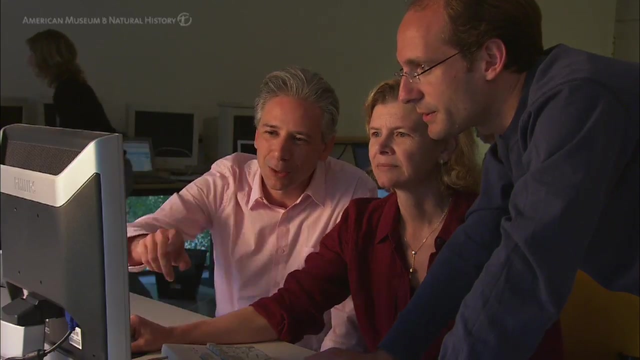 This is actually an image of one cosmic ray shower that has been recorded by the fluorescence detector. The signal that we measure is proportional to the energy deposited by the shower in the atmosphere, so to the primary energy of the cosmic ray. When you put this information together, 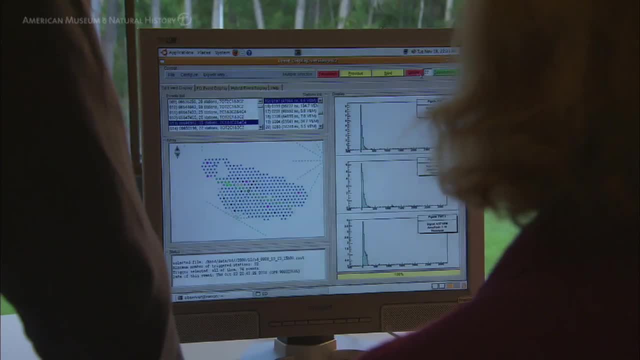 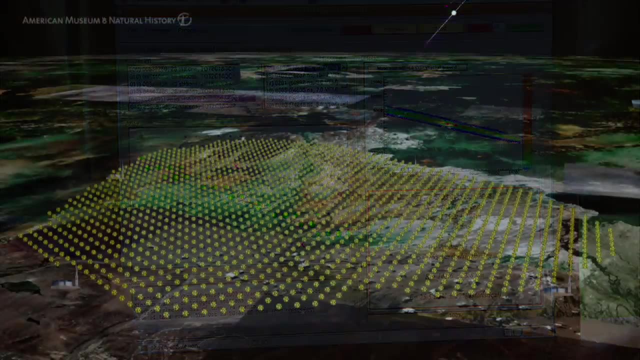 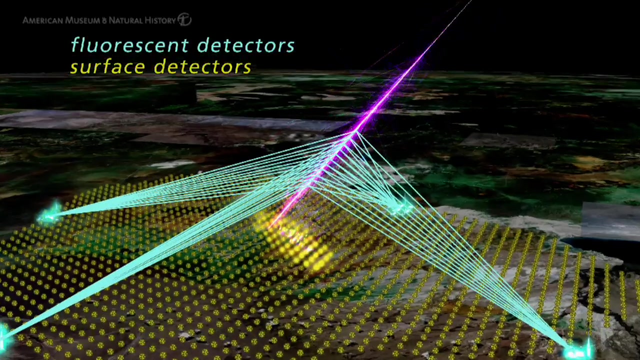 with the ground detector, we are able to explore the origin of this ultra-energy cosmic ray. Nice, that's a high energy one. Auger is finally reaching the point that we can look at where these particles actually come from, and it seems to be that they are coming. 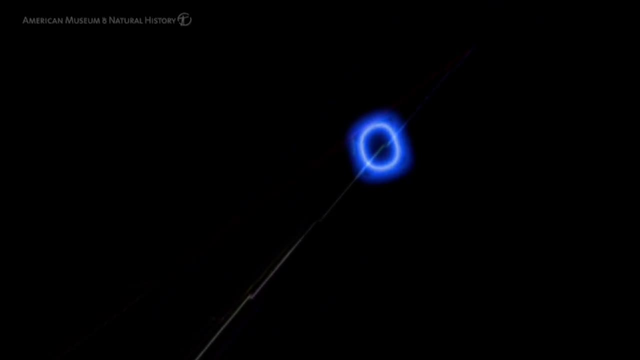 from these huge jets coming out of the centers of galaxies that we call active galaxies. Right now, we have about 30 events that seem to correlate with the positions of these active galaxies, which have a pattern in the sky that looks like the pattern that we're seeing. 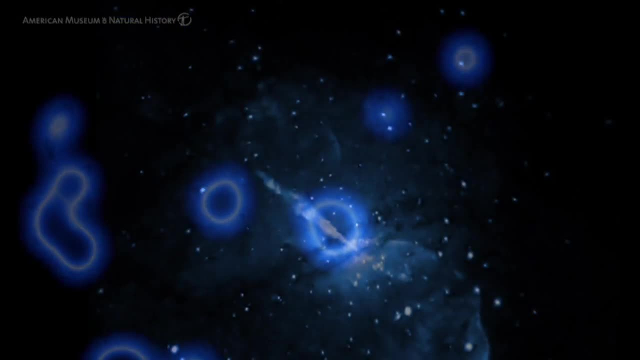 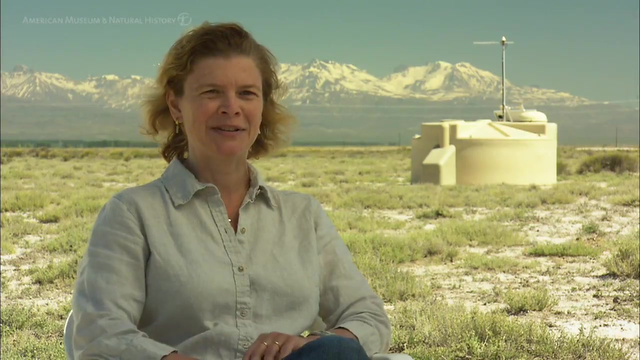 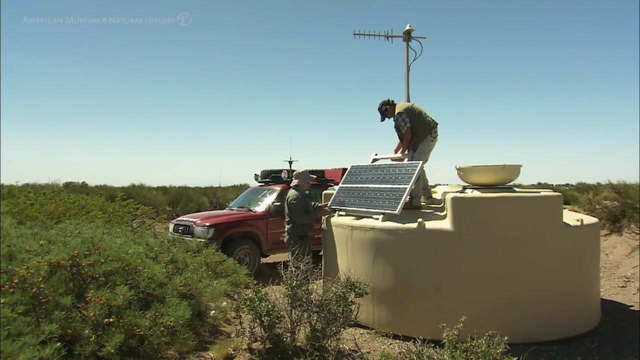 So we're starting to be able to peek at the beginning of these high-energy cosmic rays, which are much, much stronger than any accelerator we are able to build on Earth. So we're getting to the exciting point right now. I think that, touristically, 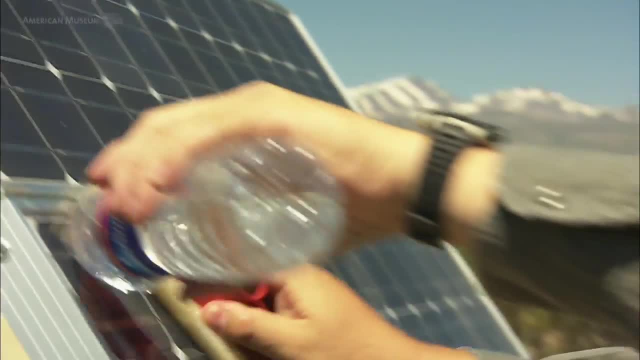 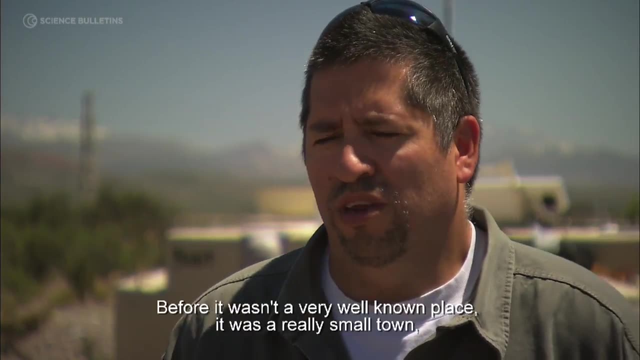 it's very useful for people. It's very useful for them. That has helped the growth of Malargue, the knowledge of the world of Malargue, because before it wasn't very well known, it was a very small town. Now it's known, let's say 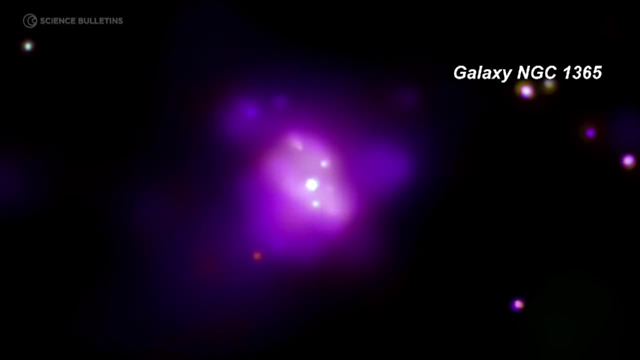 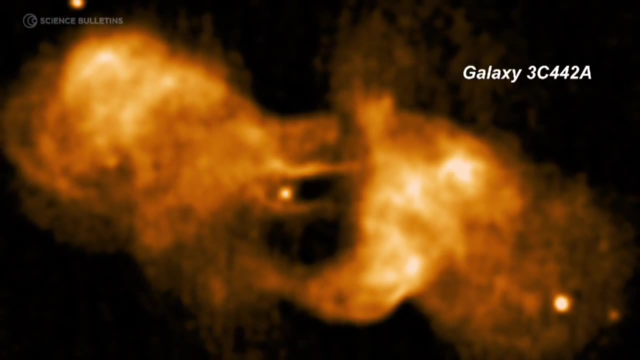 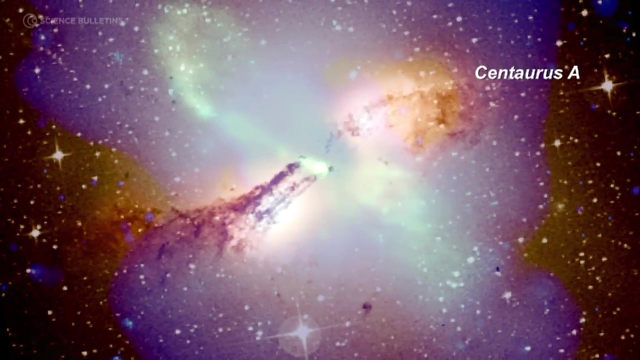 all over the world. Ultra-energy cosmic rays allow us to open a new window in the universe, a window that has never been explored before. Connecting the highest-energy particles with the universe as a whole is a very interesting quest for us, because we learn from both sides. 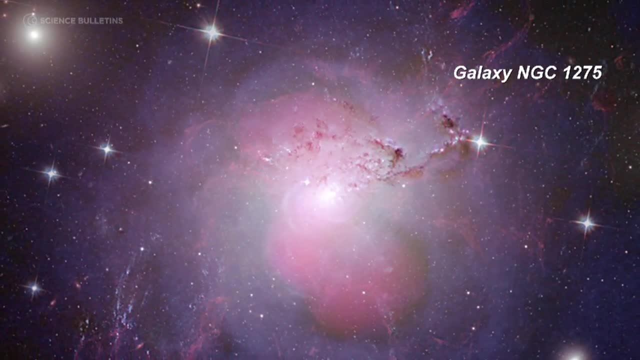 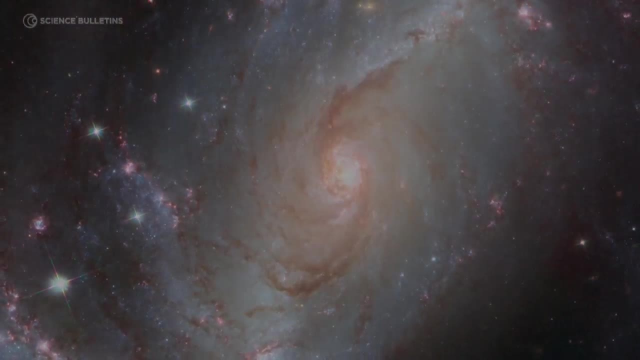 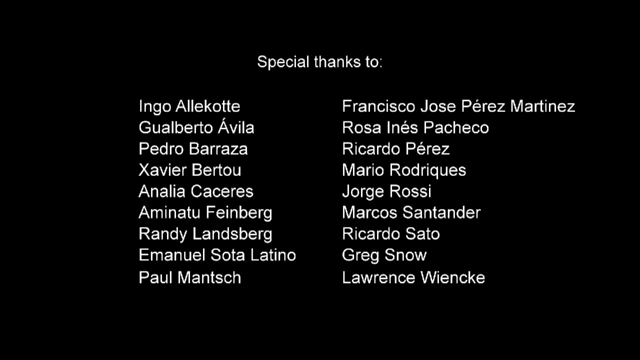 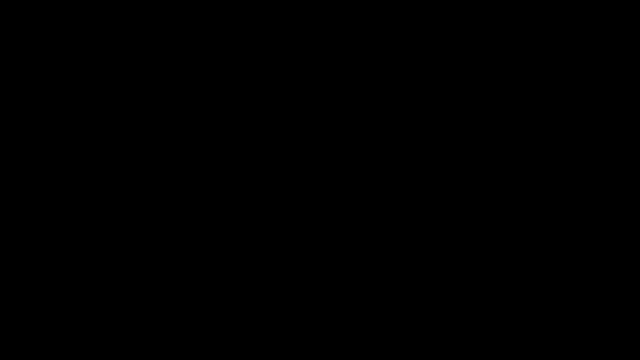 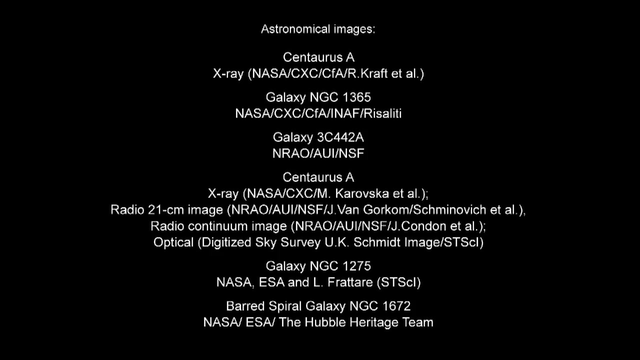 We learn how nature can produce these particles and we learn how probing these particles gives us new information about the nature of the universe. For that I'm here with this water bottle and I'm going to let it drink a drink of this water from its glass.